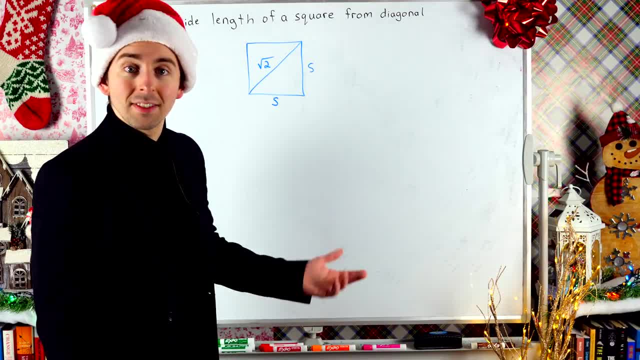 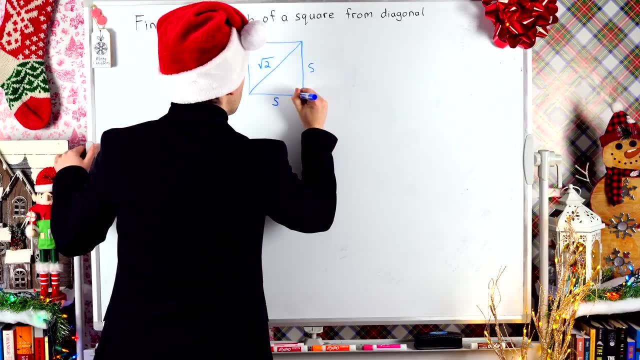 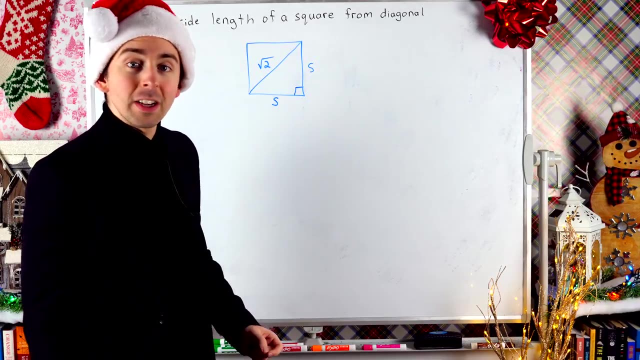 the side length, Then we'll just solve for s the side length. Well, what I notice is that here, with these two sides and the diagonal, we've got a right triangle, since the angles of a square are all 90 degrees. Now, if I've got a right triangle, certainly I can use the 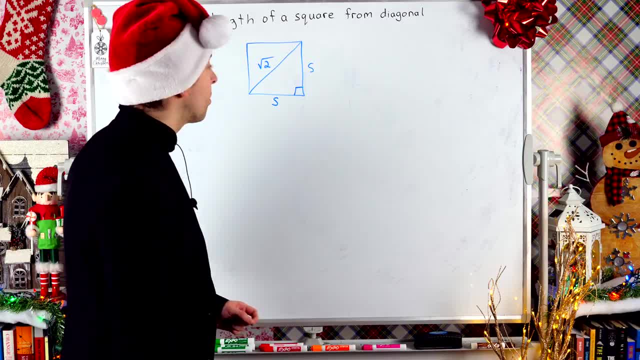 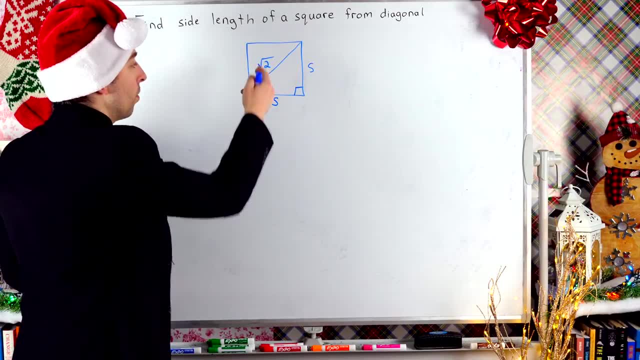 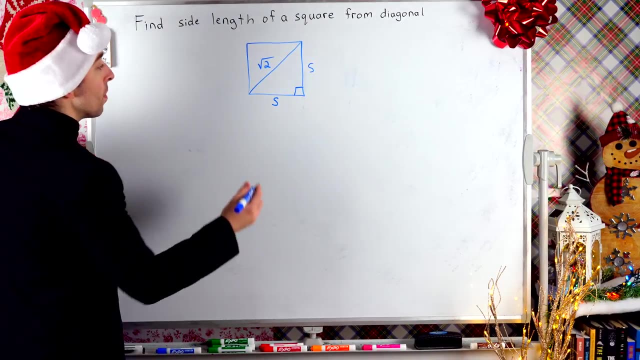 Pythagorean theorem. The Pythagorean theorem tells us that the sum of the squares of the legs are equal to the square of the hypotenuse, the longest side, which is our diagonal in this case. So let's write that equation using the Pythagorean theorem: The sum of the squares of the legs s squared plus. 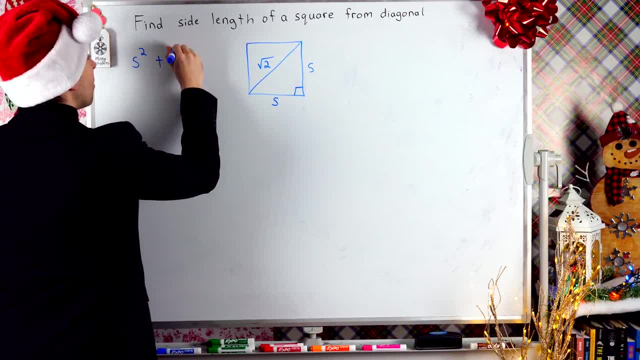 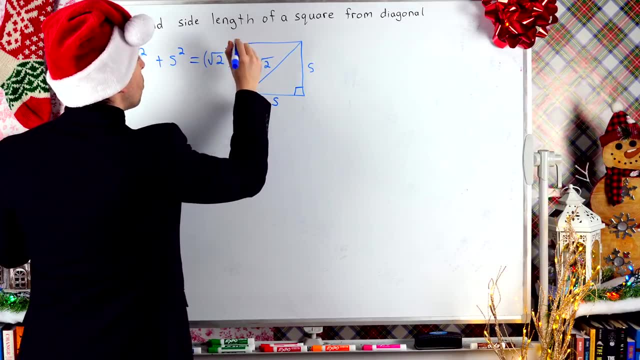 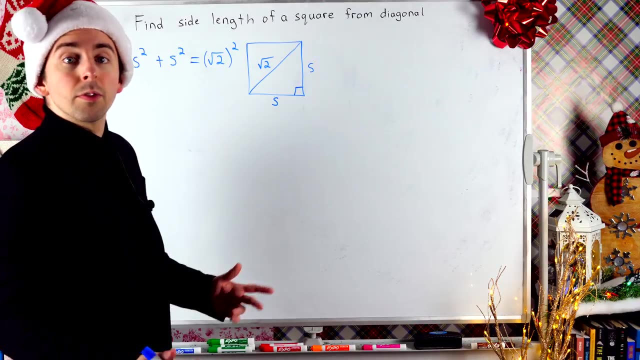 s squared, s squared plus s squared must equal the square of the hypotenuse, So that's square root of two squared Again, that's because this is a right triangle, So let's write that equation using the Pythagorean theorem. Now we've just got to solve this equation for s, s squared plus s. 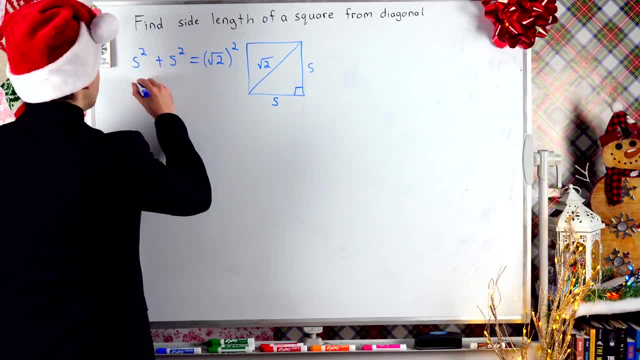 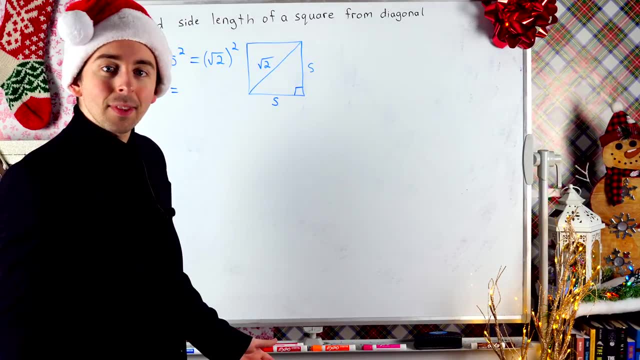 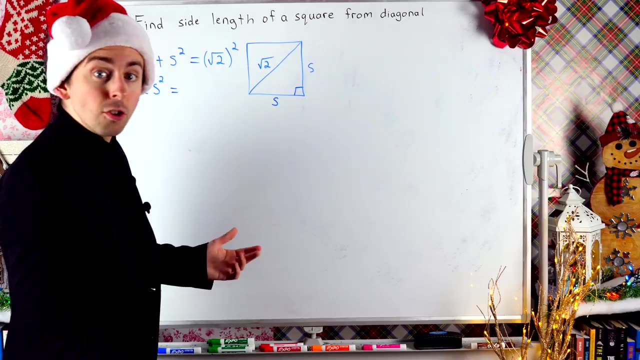 squared, that's two s squareds. So we have that two s squared equals the square root of two squared. What's that? By definition, square root of two squared is just two: The square root and the square undo each other, So this is equal to two. Now to continue getting s by itself. 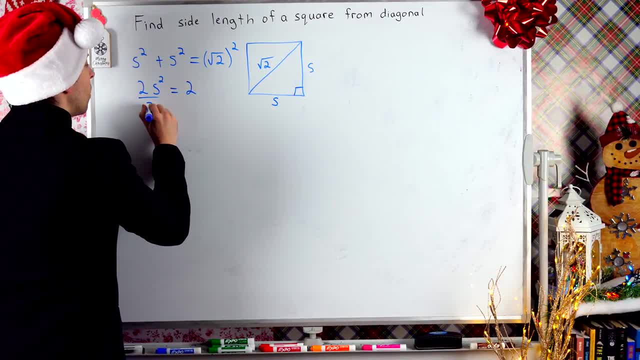 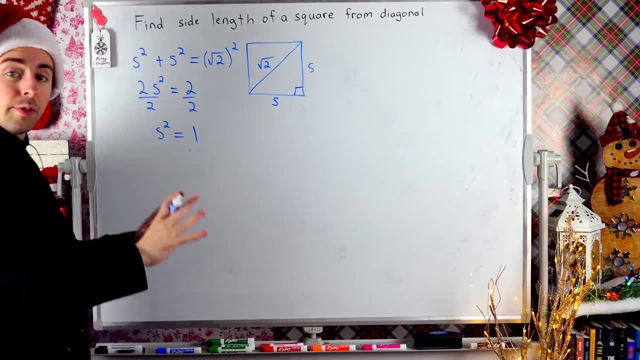 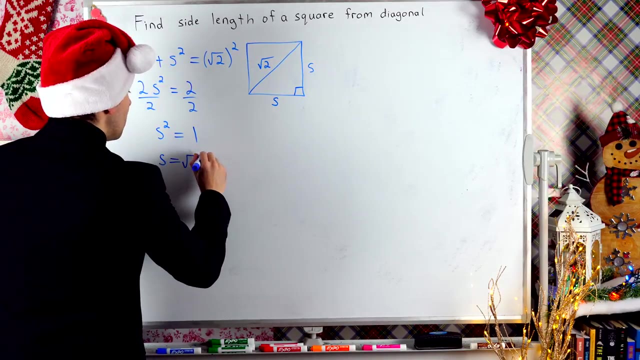 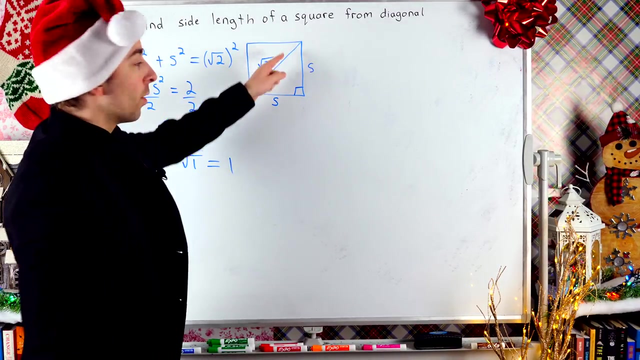 let's divide both sides of this equation by two. Then I have that s squared is equal to one. Now to finish this off, let's take the square root of both sides. So s on the left is equal to the square root of one, which is one. So the side length of this square with diagonal root two is one. I'll point out. 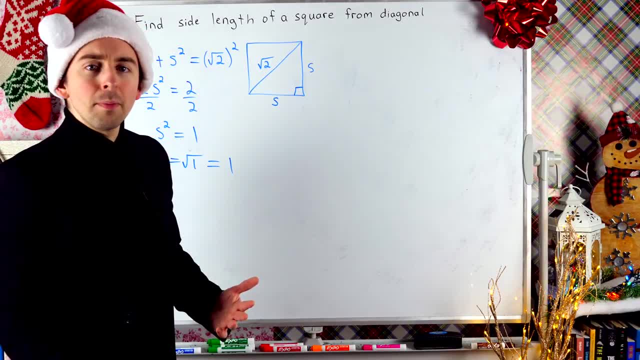 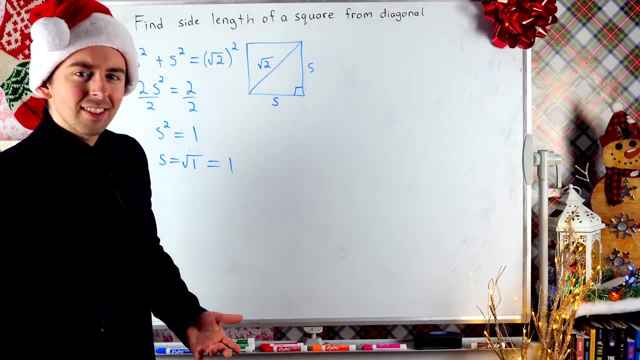 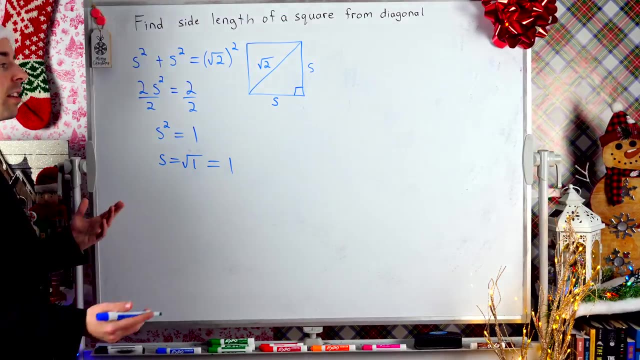 squared is 1, s could also be negative 1, but when we're talking about geometry we're not usually interested in negative lengths. we're really only interested in positive lengths. Those make sense. so we're only interested in this positive answer. 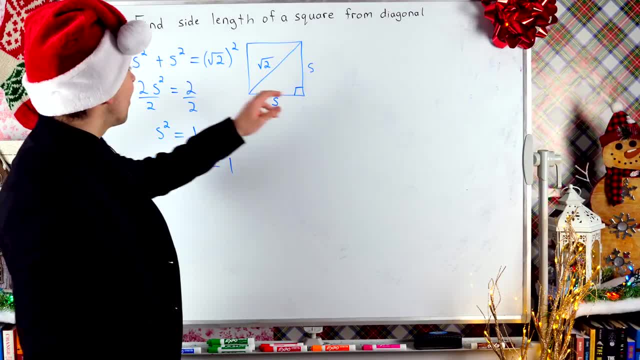 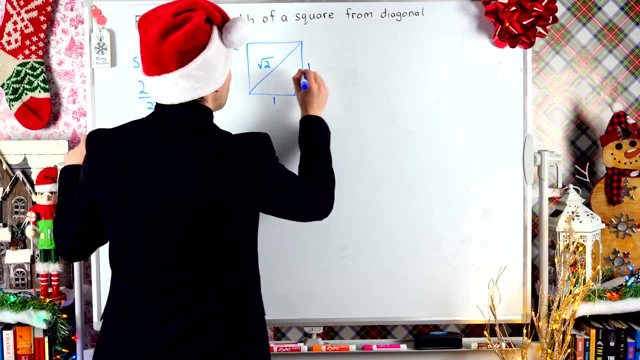 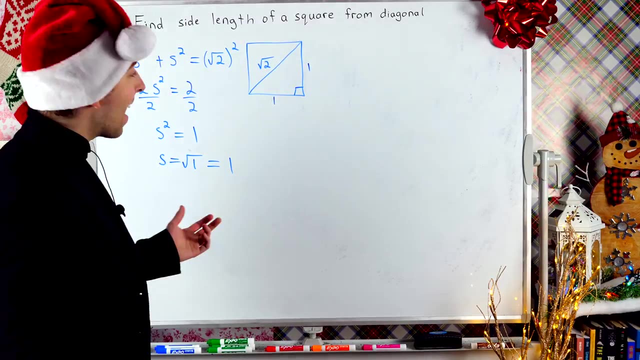 If the diagonal of a square is root 2, then its sides must all have length 1.. Pretty nice, So that's an example of how to find the side length of a square from the diagonal. but what would the general formula be so that any diagonal we have we could plug it into this? 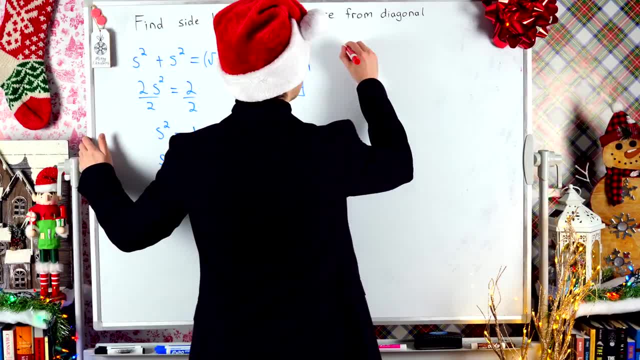 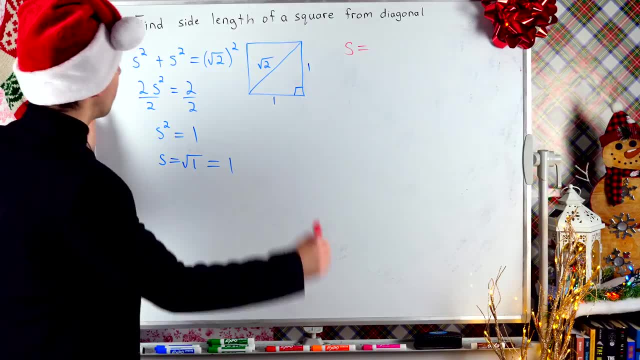 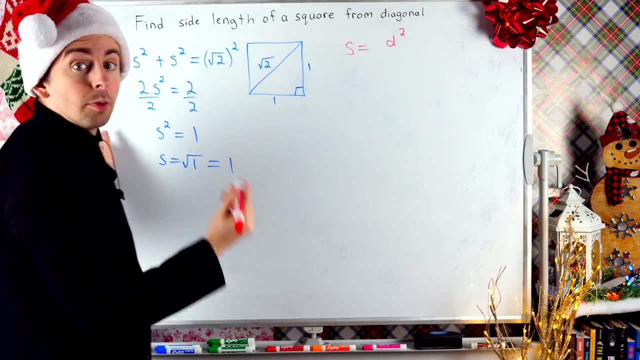 formula and get the side length. Well, the side length equals. what did we have to do to the diagonal? to get the side length? First we had to square the diagonal, so diagonal squared, but then we also had to divide it by 2, and then, to finish things off, we had to take a square root. 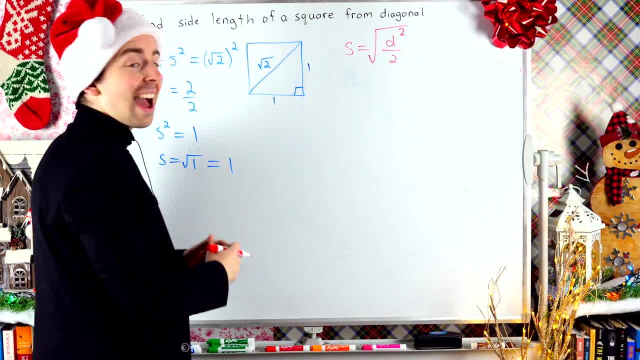 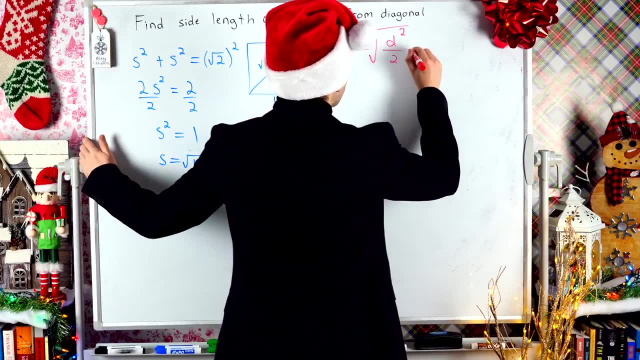 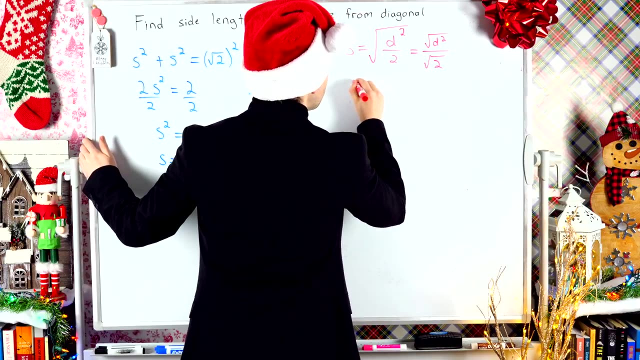 So in general, the side length of a square with diagonal D is the square root of D squared divided by 2.. Now we could rewrite that as the square root of D squared divided by the square root of 2, and the square root of D squared is just D, so that's equal to. 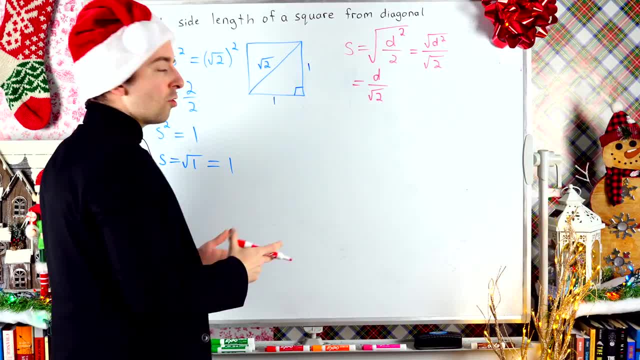 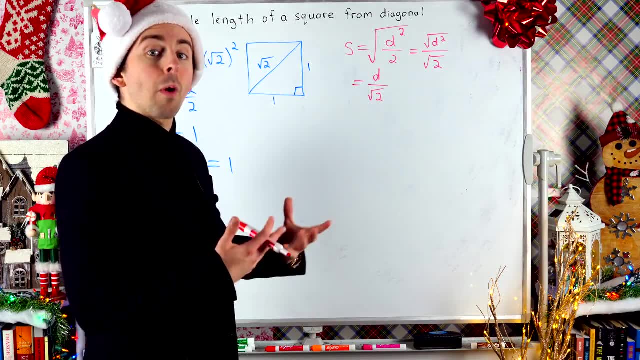 D squared divided by 2.. over the square root of 2,. and then it's generally considered better form to not have square roots in the denominator. This is called rationalizing the denominator. In order to get rid of that square root of 2,, we'll just multiply by: 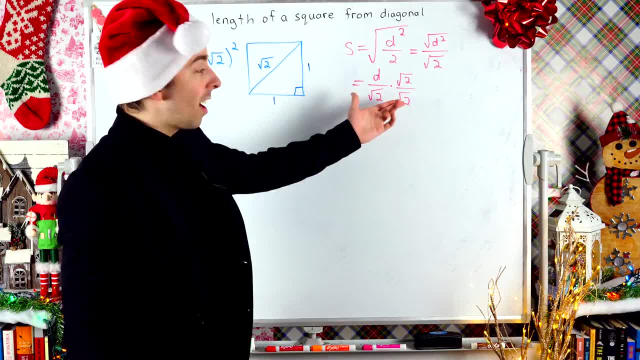 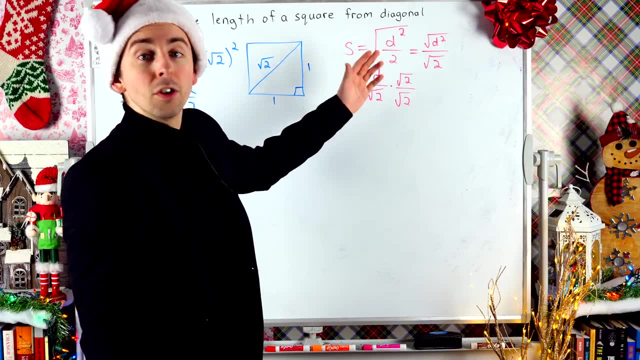 root 2 over root 2.. That's the same as multiplying by 1,, so it doesn't change the value of the expression, but it's going to move the square root to the numerator instead of having it in the denominator. So what we'll have is D. 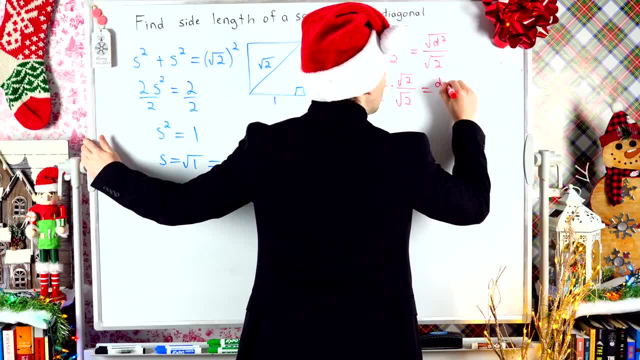 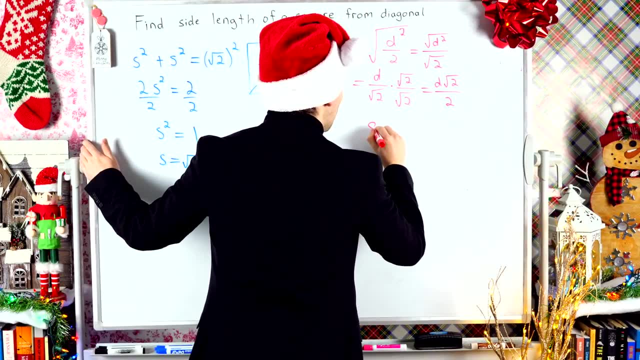 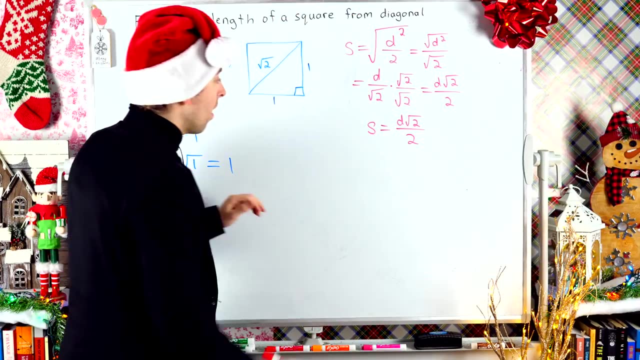 times the square root of 2, so D root 2.. In the denominator root 2 times root 2 is just 2, and this could be our final formula: If a square has diagonal length D, then its side lengths are D times root 2 divided by 2.. Pretty nice, but really. 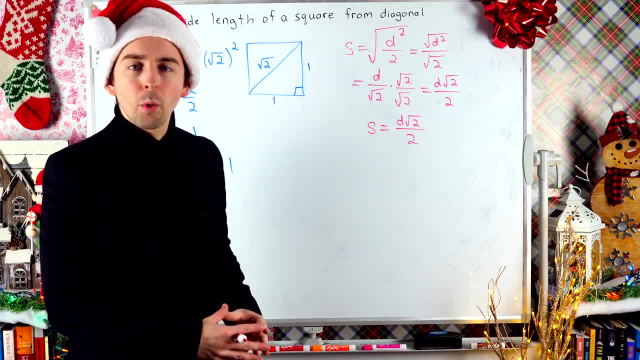 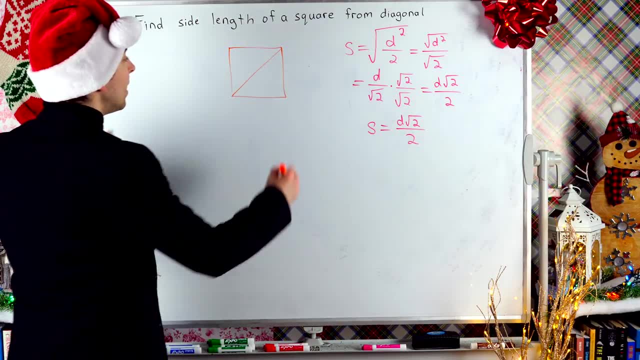 the process is so simple that you can't do anything about it. Let's do one more quick example. So here I've got another square. Let's say its diagonal length is 5, and again I'm trying to figure out the side length of the.